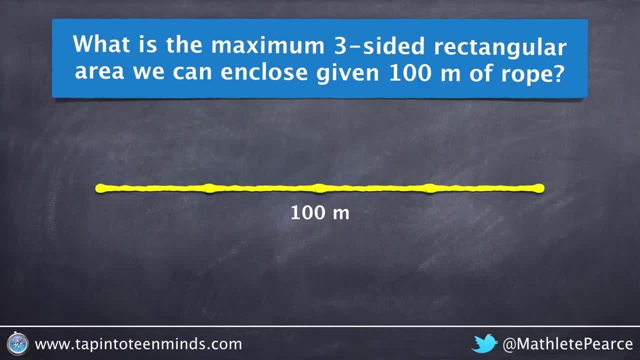 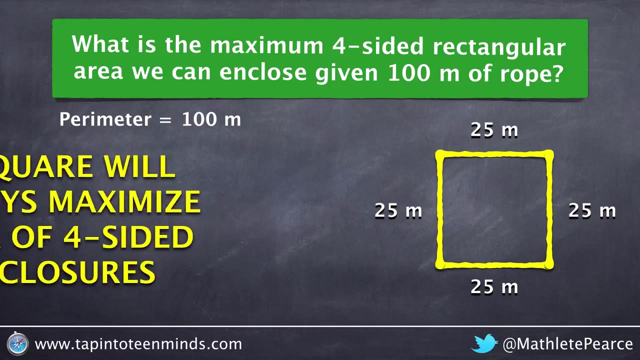 Let's take a few moments to explore the maximum area for three-sided enclosures. In this case, we'll be given 100 meters of rope to work with. Recall that the area of a four-sided rectangular enclosure could be maximized using a square, So in this case that is a 25 meter. 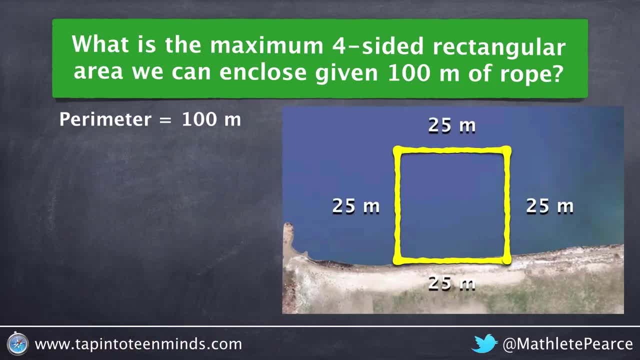 by 25 meter square. However, in some situations we don't need four sides to enclose the rectangle. For example, if we're at the beach and we're looking to rope in an area to swim, we don't need to rope. 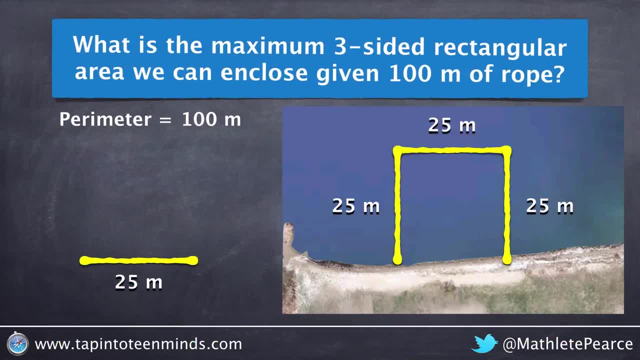 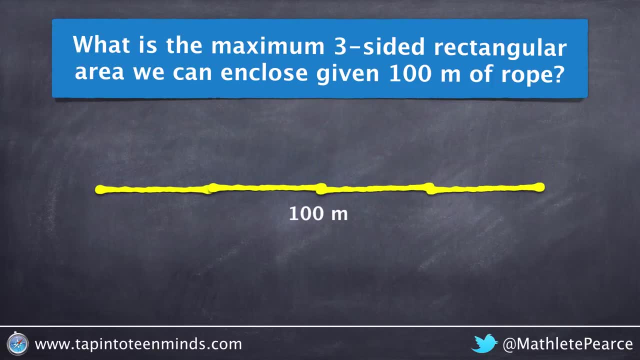 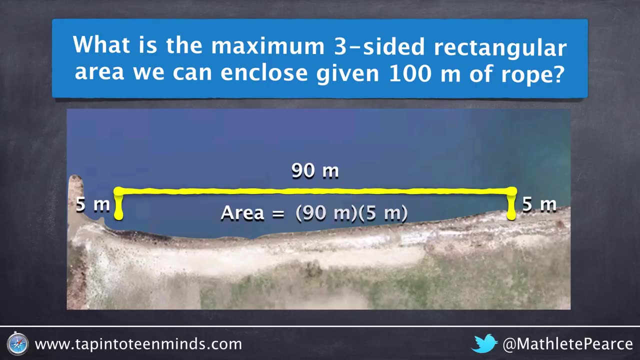 off the side along the beach. So we would be left with two widths and one length to work with. So what should we do with that fourth side? We could start with a very narrow swimming area, as we did in the four-sided case, but, as we remember, that doesn't yield a very big area Relating width to 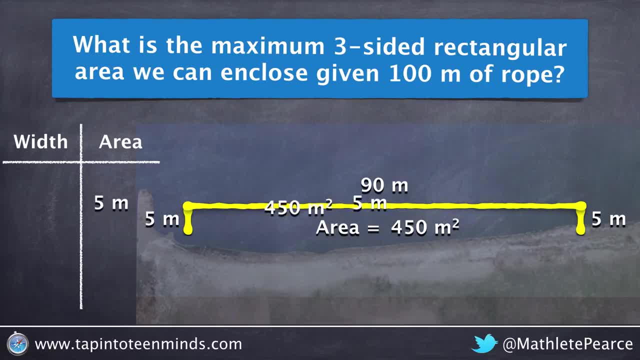 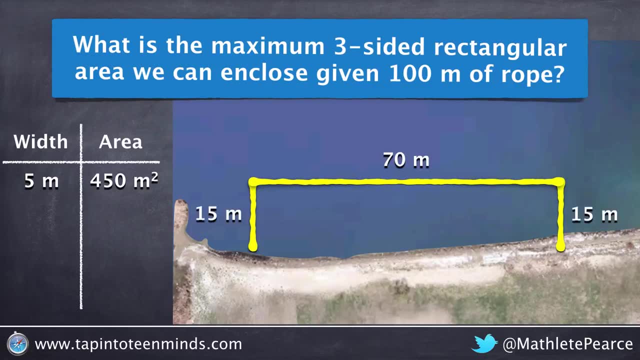 area. we can see that the area of the four-sided enclosure is a very small area, So we don't need that. The width of five meters will yield only an area of 450 meters squared. Increasing our two widths to 15 meters each, we can see that we'll have 70 meters left of rope for our length and 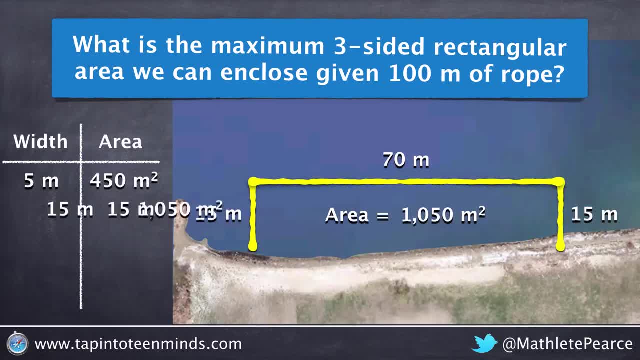 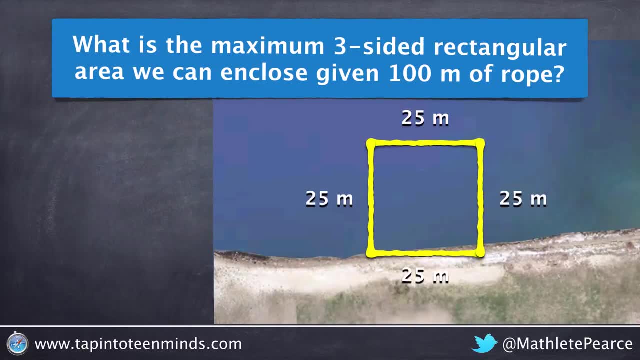 our area to swim will increase to a total of 1050 meters squared. Now many of you must be sitting back and thinking: why don't we go back to the square idea that we used for four-sided rectangular areas? If we took that extra side and we split it up amongst the three sides of our enclosure, we could 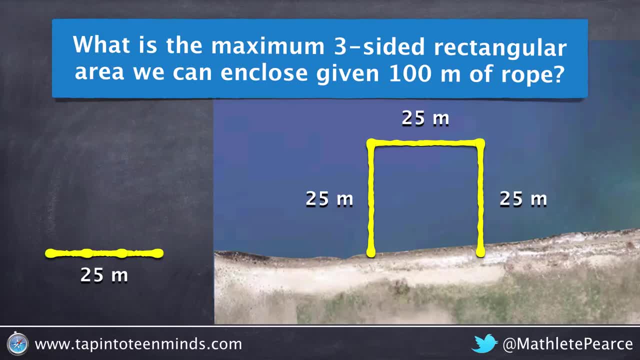 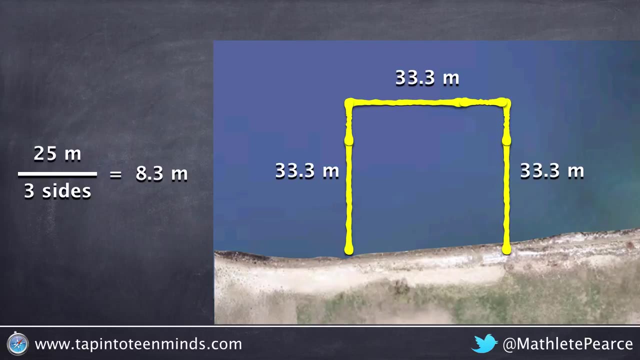 get a larger rectangle and thus have the maximum area. So, dividing 25 meters by the three sides left, we end up with 8.33 meters to add on to our two widths and our one length. So let's take a look and see what that does to our area. Multiplying 33.3 times 33.3, or squaring, 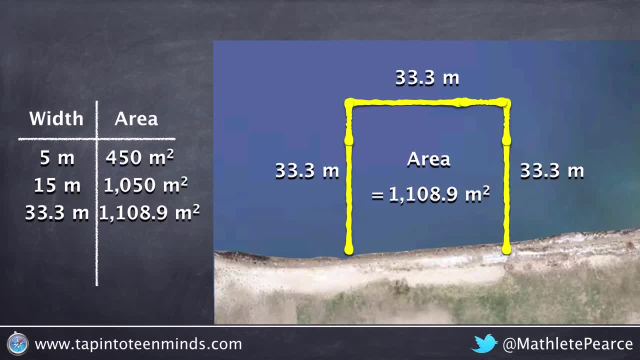 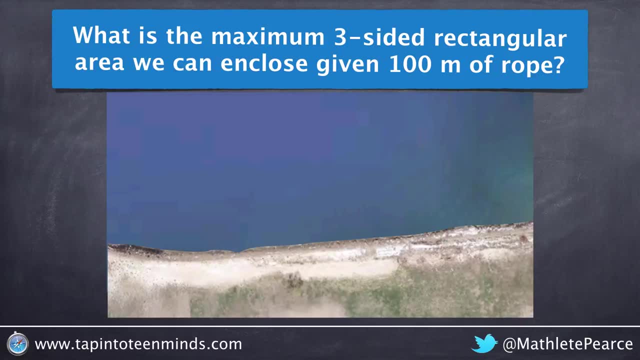 33.3,. we end up with a total area of 1108.9 meters squared. Now, while this is better than what we've seen so far, surprisingly it is not the maximum area for a three-sided enclosure. So let's go back.